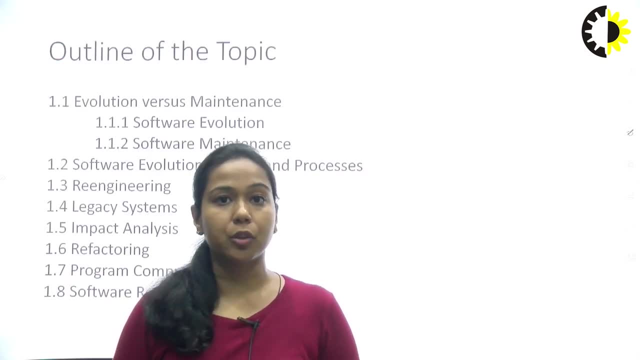 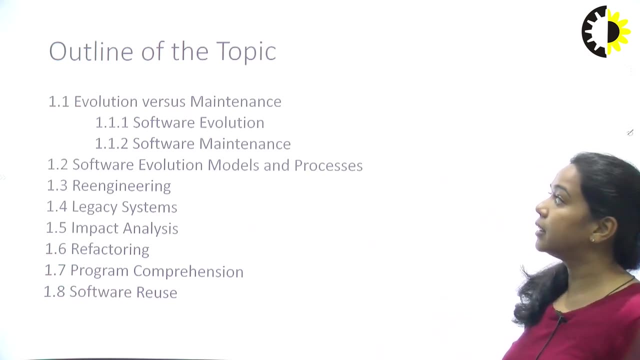 in a software engineering, in a software development complete process. So what are the outlines we will going to be cover in this session? that first of all we will going to cover, that is, the evolution versus the maintenance In the sub part of the evolution versus maintenance. 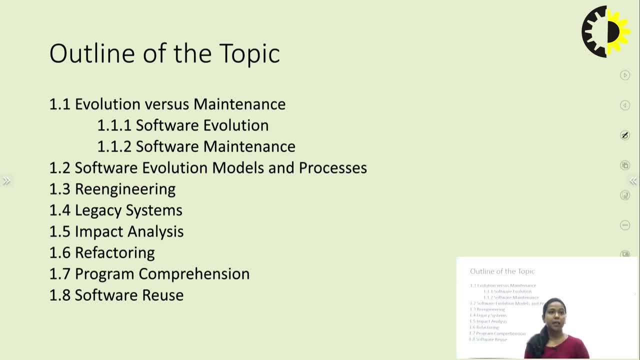 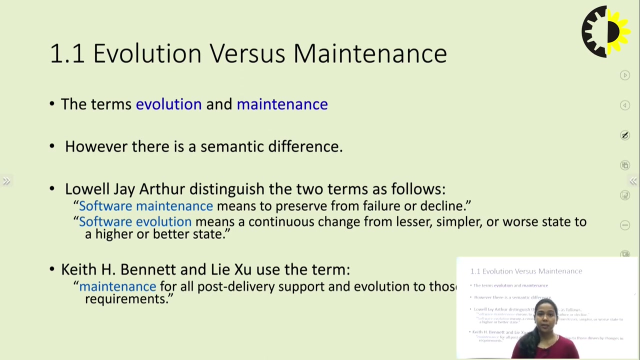 is the software evolution and the software maintenance, The software evolution models and their processes, the re-engineering and the legacy system, impact analysis, refactoring and program comprehension. Lastly, we will going to be discuss about the software reuse. Now, what is the actually difference between the evolution and the maintenance? Why we 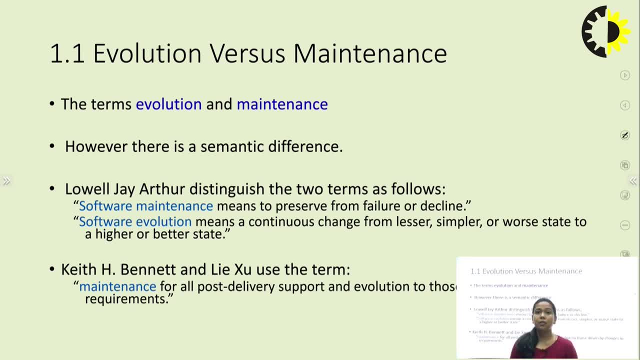 are discussing about at the initial phase. we are discussing about the evolution of the software, that how the software will going to develop, how the processes will going to be make up. Later on, we are end up with the maintenance phase, which will be the never ending process. So what is the difference between both of these terminologies? that is, 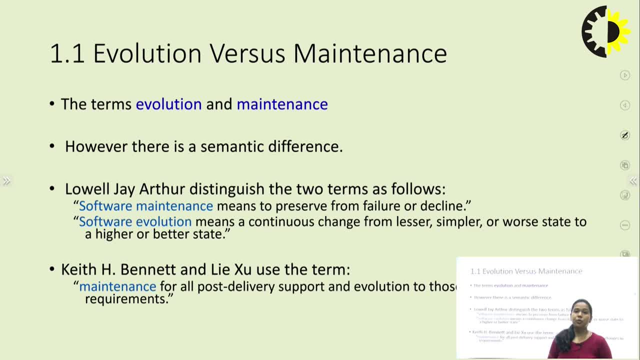 the evolution versus the maintenance, The term evolution and the maintenance. however, there is a semantic difference between them. The Lowell J Arthur distinguish the two terms with the help of their definition given by them: Software maintenance and the software evolution. Software maintenance means to preserve from. 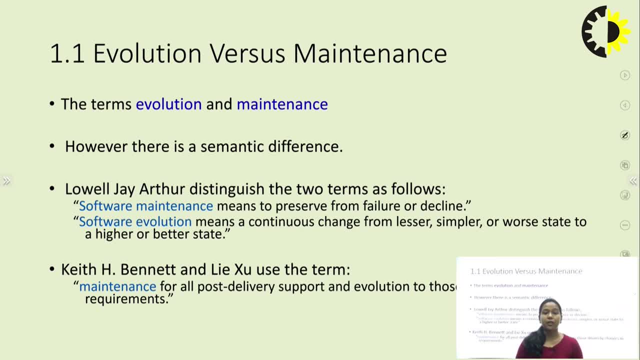 the failure to the decline. This is the maintenance phase where we are trying to preserve the failure to the decline. If the failure will come, the fault will occur in a software. we are making them preserve that it should not be reached to the decline phase that we need. 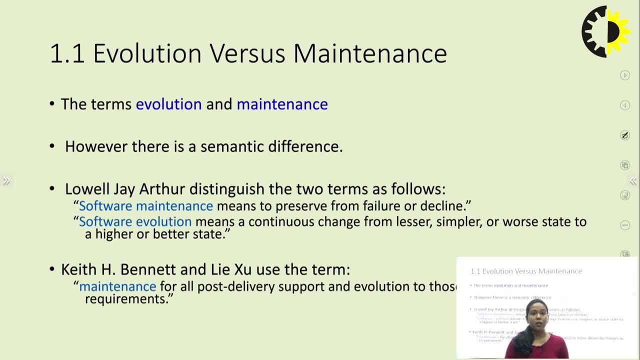 to be dump that software. We are not reaching to that phase of the software, Whereas the software evolution means a continuous change from the less than to the increase in the failure to the decline phase. So the software evolution means that we are continuously doing. 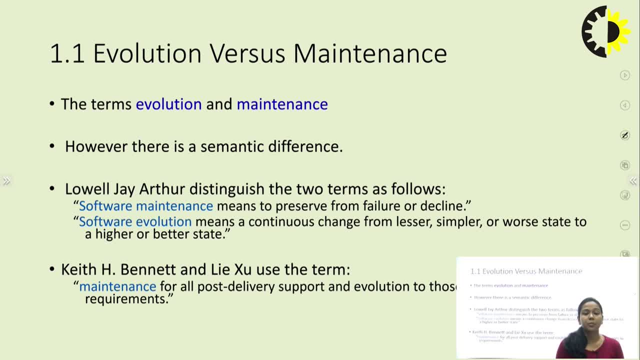 the processes and making the software in such a way that it can be easily, that it can be simplified, used by the user. The user is comfortable to make them use. that is the state which will be going to be done in a software evolution, Whereas the Keith H Bennett and the Lee Zhu. 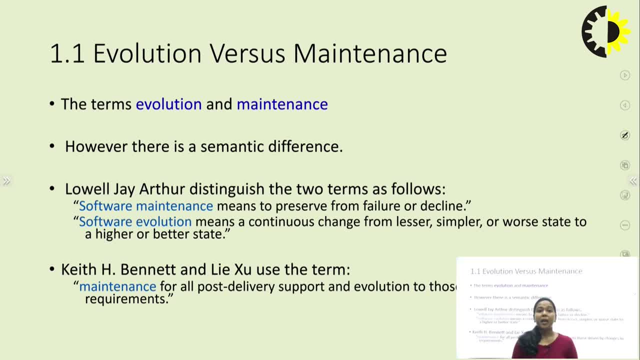 use the term maintenance, Maintenance for their post delivery support and also the evolution will be given by the change in the requirement. That means the changes will be come in a requirement that will be give a evolution of the next version of software, Whereas the maintenance will. 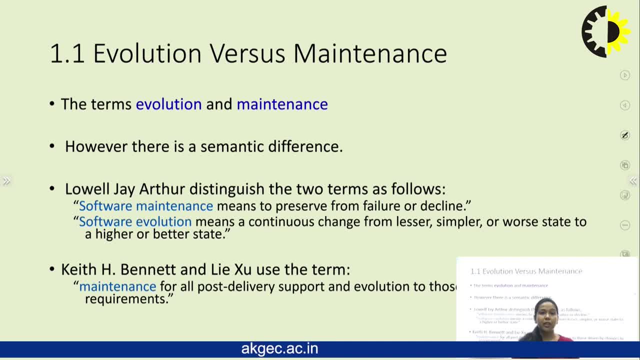 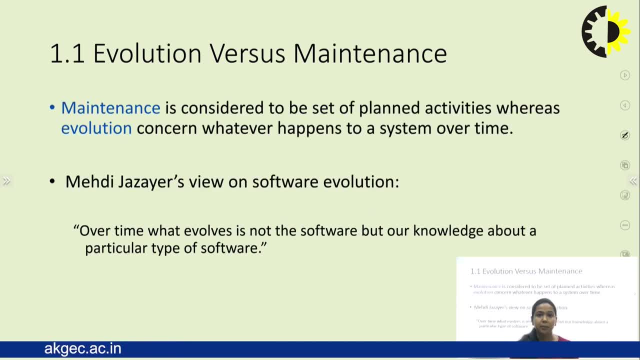 be the continuous process of making the software not reaching to the decline state. Make them usable by the user as per the requirement given by them. Now the maintenance is considered to be set for the next version of the software. So the maintenance is considered to be set. 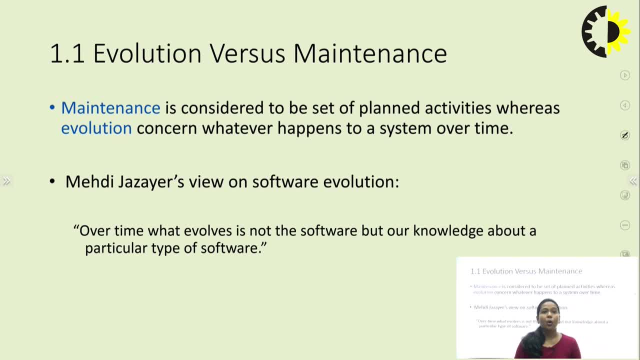 for the next version of the software. Now the maintenance that the development of software evaluation. So the maintenance is considered to be the set of the plant employees as per the requirement for that. That means the maintenance as regard to Vehicle basic viewers experience, the contraction of the software which is been planned Thenそれは. 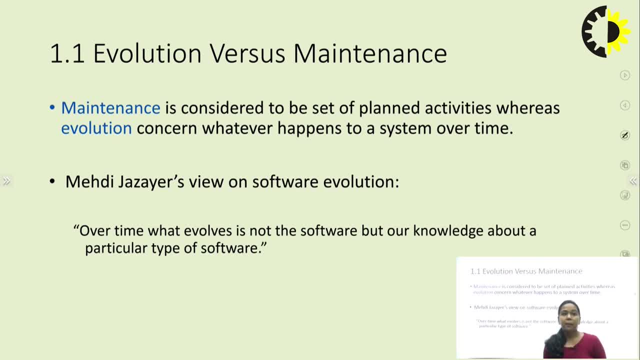 being done. software evolution, the Mehndi they serve, viewer software evolution, that is, over time. what evolve is not a software but over knowledge about the practical, particular type of software, the overtime. we are not actually evolving the software on the basis of the knowledge. the changes we will going to be cover up. 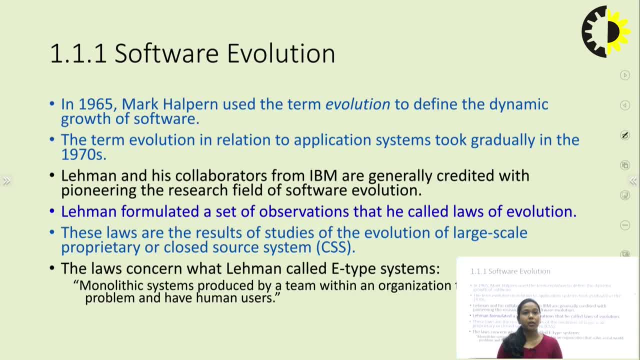 is known the reach of the evolution of a software. so in 1965 the mark helper use the term evolution to define the dynamic growth of the software, where the term evolution is relation to the application system, to they gradually in the 1970s, whereas the layman and his collaborators from the IBM are generally credited with. 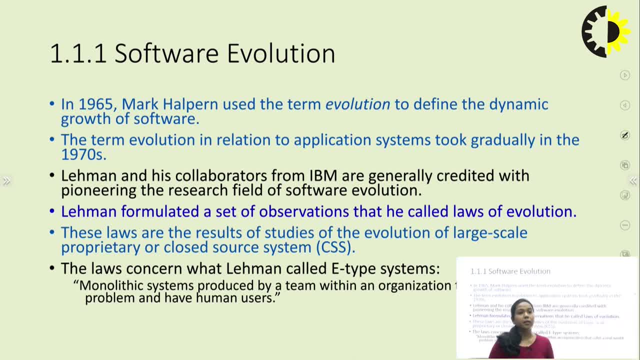 the pinering, the research field of the software evolution. the layman formulated the state of observation that he is called the law of evolution. these laws are the result of studies of the evolution of the largest scale, not on the smaller scale. they are actually evaluating or evaluating the software. 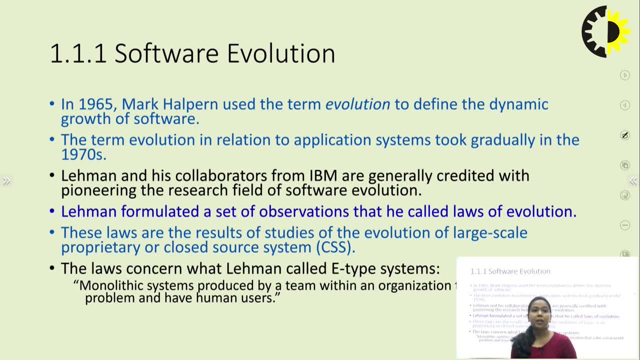 their evolution on the large scale it to be happened. the law concerned what layman called e-type system, the monolithic system produced by a term within the team with an organization that solve a real-world problem and have a human use. that is the law which is given by the 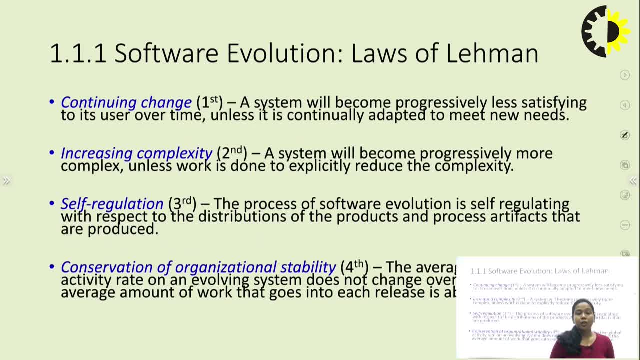 man, the software evolution, given the certain terms, which is explained by the layman as a law of the layman for the software evolution to be explained. so continuing changing first of all, a system will become a progressive less satisfying to its user over the time, unless the continual adopted of meeting. 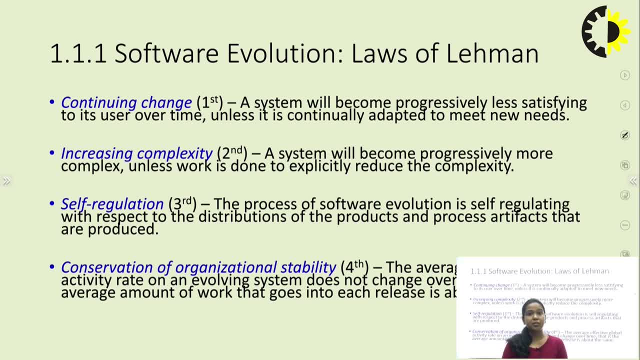 the new needs. we are trying to progressively less satisfying the user if they're actually continuing changing their requirement as per the their attraction or as per the their interaction or as per the their satisfaction toward their system or their software, increasing the complexity. secondly, if the complexity increases, the 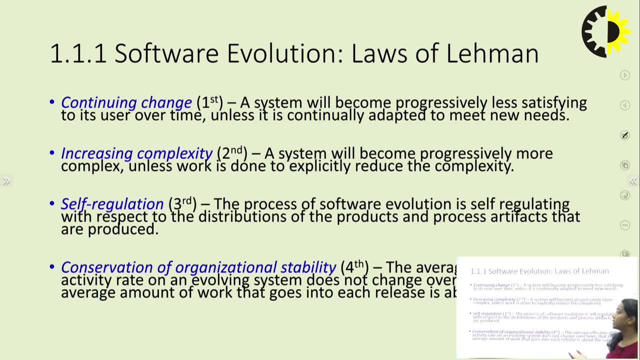 system will become progressively more complex unless the work is done explicitly reduce the complexity. self-regulation: that means the process of software evolution is self-regulating with respect to the distribution of the product and process artifacts that are produced. conservation of the conservation of the organization's 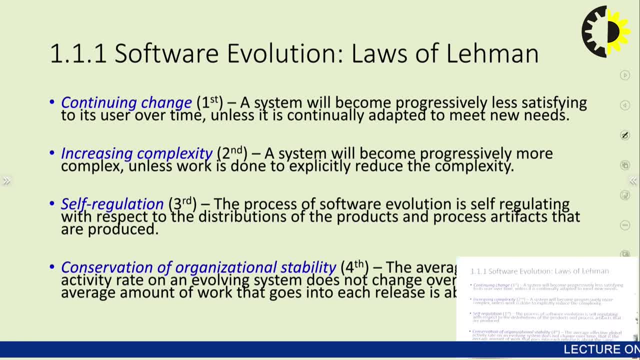 stability, the average effective global activity rate on the basis of evaluating the evolution of the software. it does not evaluated own the basis of the of at a time. that is the average amount of the world that goes into the each release. that will be the above case in this. so these are some of the laws. the 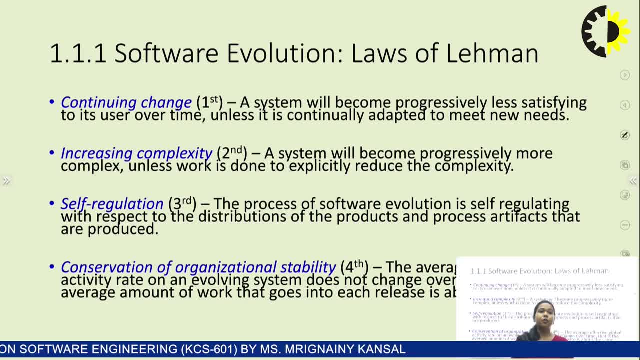 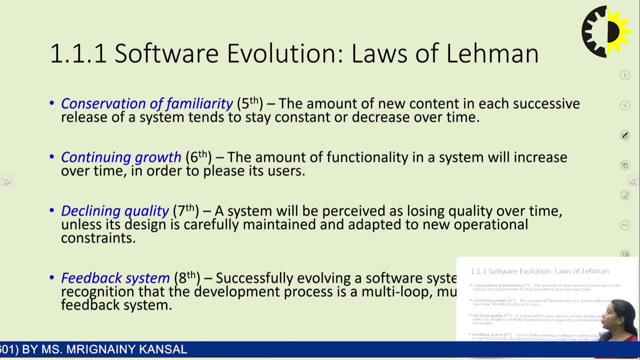 the four laws here. it is explained in the next slide. we will going to be understand that. what are the other laws given by the layman? the fifth one, that is the conservation of the familiarity that means the amount of new content in the each successive release of the system tend to stay constant and 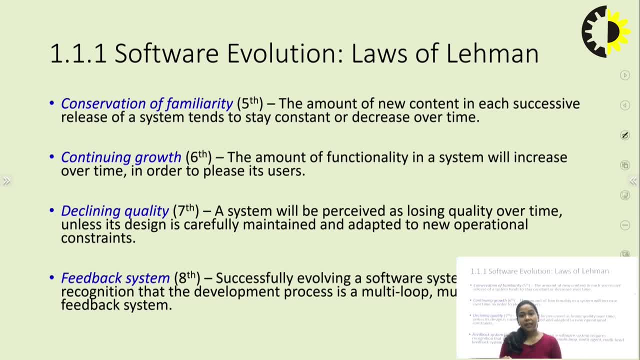 decrease over the time. that will be decreased at the iteration. the amount of changes to be done get decreases because continuously we are actually doing the effort in the evolution of the new software. evolution in the software will reach the customer to their satisfaction. continuing growth, the amount of 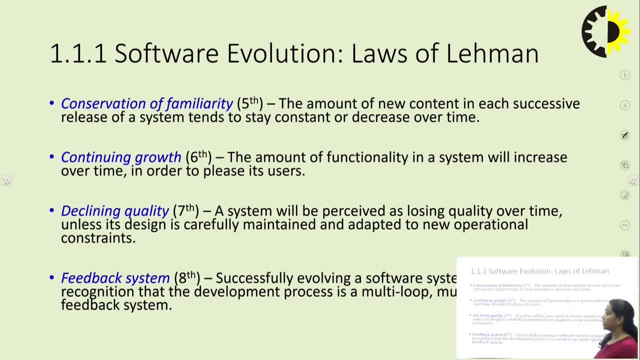 functionality in a system will increase over the time in order to please its user, declining the quality. a system will be perceived as losing the quality over the time unless it designed it carefully and new constraint will become as per the time move on further. lastly, the feedback system. the feedback will help the developer to 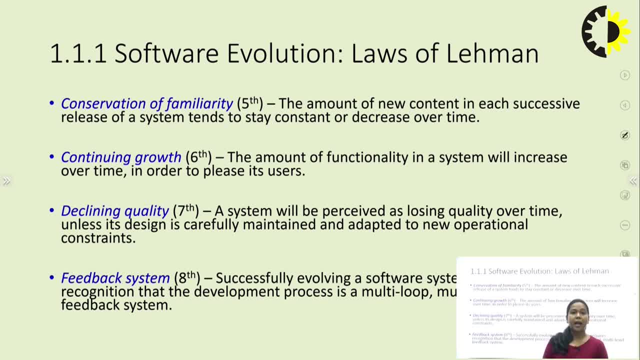 understand the actual requirement of the user. the user, when interacted with the system, will provide their feedback that what actually they are getting from this so successfully involving a software system, requires reorganization. that the development process is a multi-loop, multi-agent, multi-level feedback system. that means at every successive level, at the every. 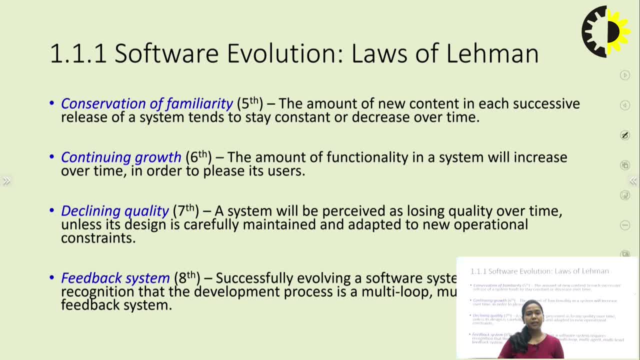 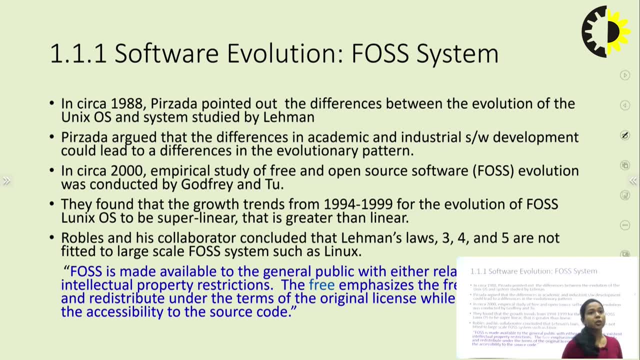 level. we are getting the feedback from the customer and get to know the feedback from the user and get to know that actually what they are want, what they are actually required from the system. now the evolution on the basis of fo SS, that in the case on 1988 the pointed out the difference between the 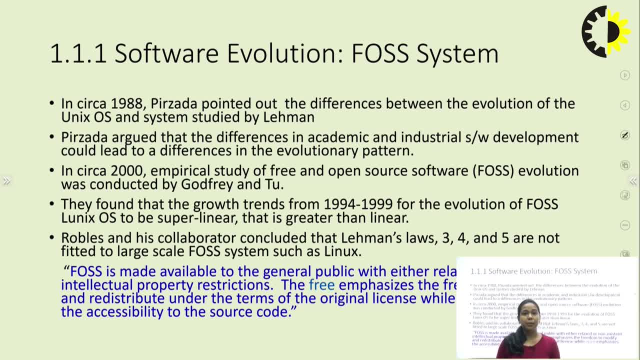 evolution and the Unix of OS and the system studied by the layman, the. what is different between the laws which is given by the layman, as well as the Unix OS which is currently used in a market? so they are arguing the difference in the academic and the industrial software development could lead to the difference in the evolution. 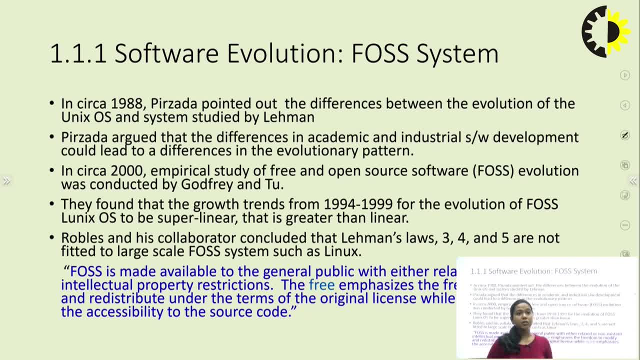 pattern that how it is evolving. the seka 2000 empirically studies of the free and open source software evolution was conducted by the godfrey and the two. they found the growth tend to be 1994 to 1999 and for the evolution of the post linux os to be the super liner that is greater than the. 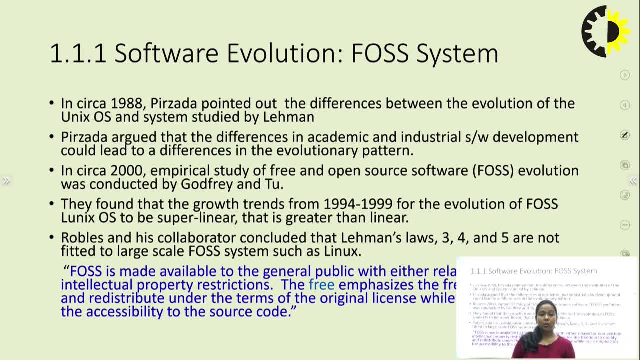 liner the robles and his uh corp collaborator concluded that the layman laws of three, four and five are not fitted to the largest scale force system, as like the linux. so the force is made available for the journal public with either to be the relaxed and the non-existence intelligent. 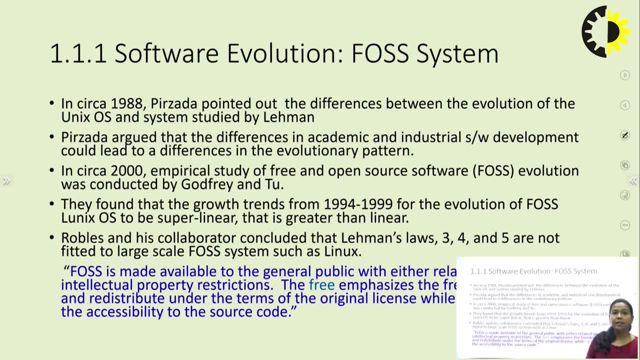 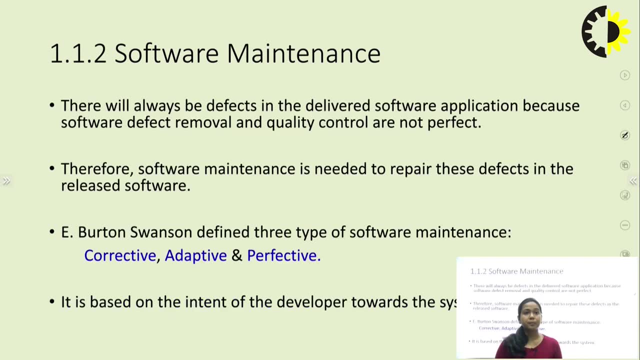 about the property of restriction and free emphasis, the freedom and the redistribution over the term of the original license, while the open emphasis and the accessibility of the source code. this is the providing of the definition of f? o table as false. now we have discussed uh layman laws and the false criteria or the 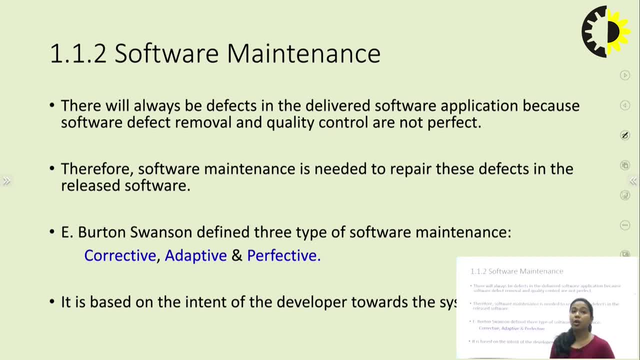 point of view about the software evolution. now we come out with the topic that is, a software maintenance. there will always be defect in the delivery software application because the software defect removers and quality control are not actually the perfect personality to be done in the previous state of your software development process. 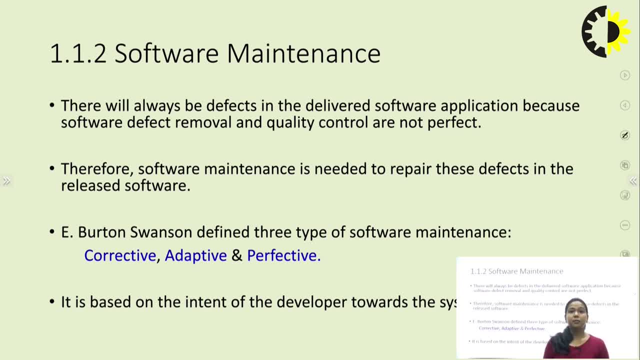 so therefore, the software maintainances need to be repaired and these defect in the released software. so a burton swithsome defined the three different type of the software maintenance on the basis of corrective, adaptive and the perfective way they are defining the software it is based. 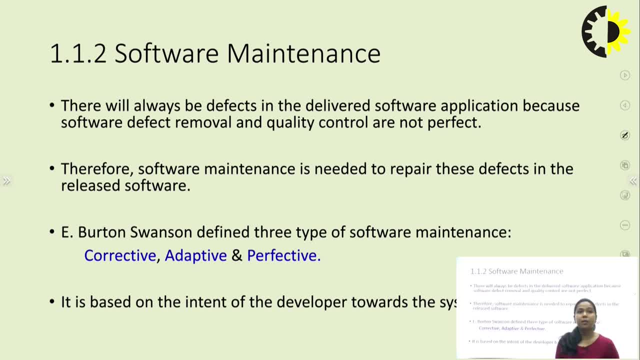 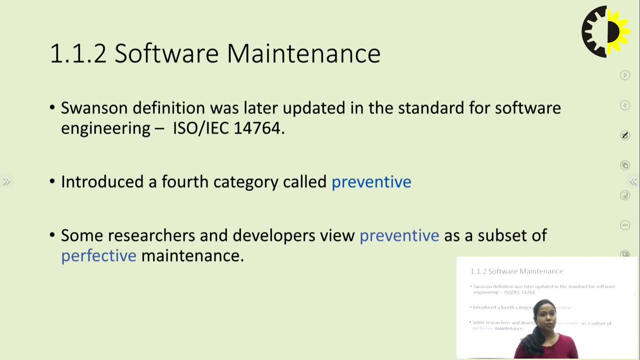 on the intent of the developer toward the system. this is the software maintenance. the swenson definition was later updated in the standard of the software engineering that is. iso introduced a fourth category which is known as the preventive, and some researchers and the developer view perspective as a subset of the perfective maintenance. this is done by the help of the 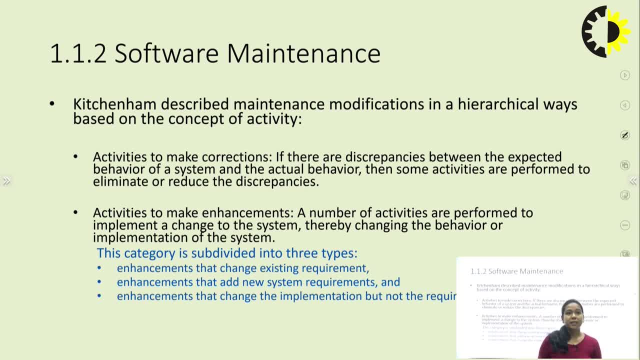 software maintenance. the kitchen hem described the maintenance modification in a hierarchical way based on the concept of activity. activity to be make the correction of their are the discrepancies between the expected behavior of the system and the actual behavior. then some of the activities are performed in eliminating or reducing the discrepancies. so the 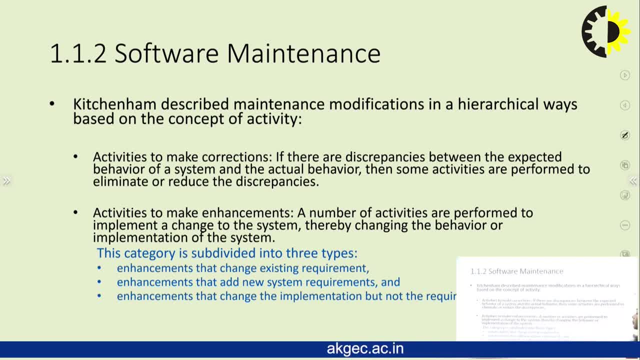 activity to make them enhancement. a number of activities are performed to implement a change to the system, so thereby changing the behavior implementation of the software to be done. so there are some of the subcat division of these three part. on the basis of enhancement, that change exists. the 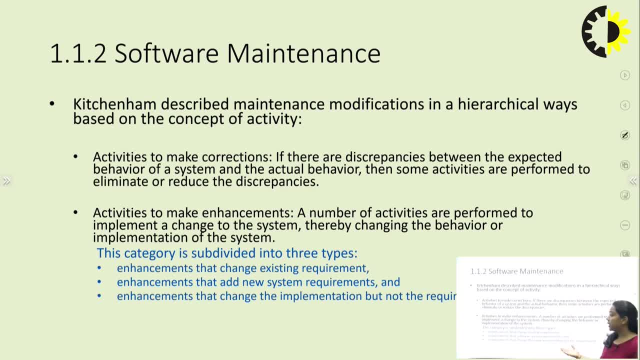 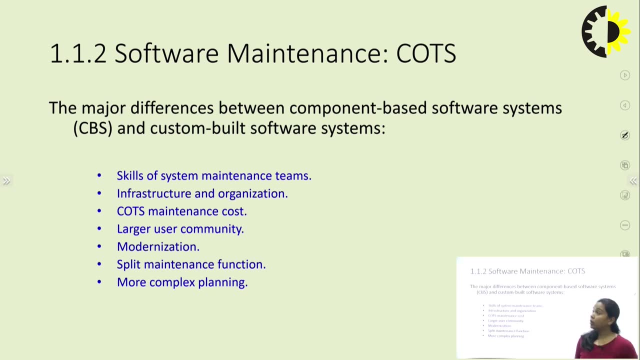 on the basis of enhancement that add the new system requirement and on the basis of enhancement that change the implementation but not the requirement. so these are the three subdivision of the category which is explained in the software maintenance. now we will going to be define the maintenance on the basis of the courts, the major difference between the component based. 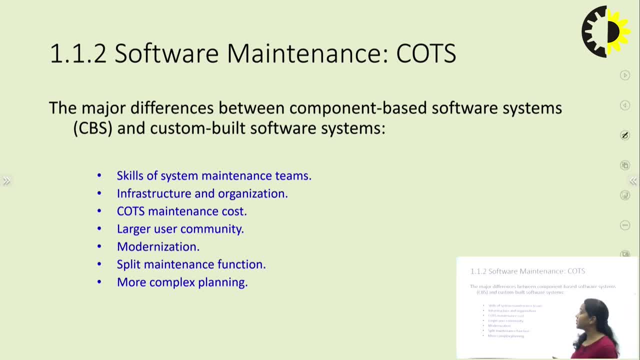 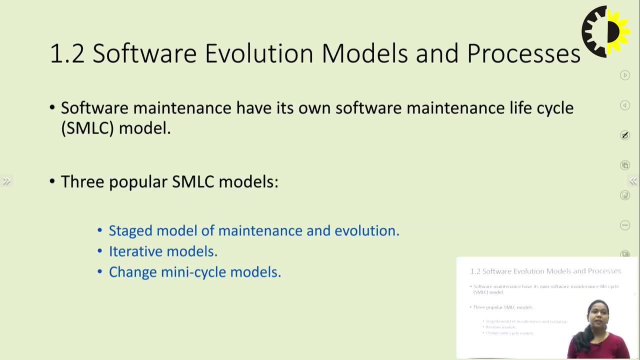 software system and the customer built software system are on the basis of skill of the system maintenance team, on the basis of infrastructure and organization, court maintenance course, larger user community motorization, split maintenance function and more complex team. now the software evolution model, the second topic. we will going to reverse that. what are the model which is used for? 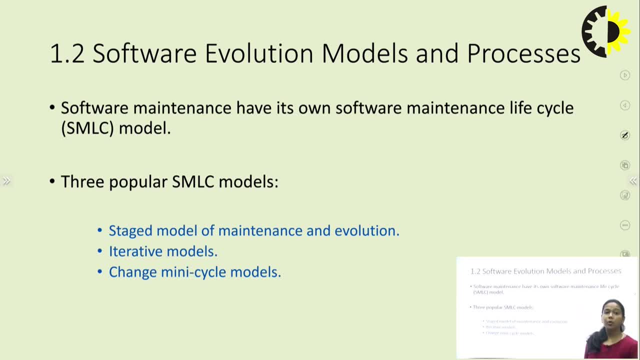 the software evolution. so first of all we will going to be use the software maintenance of their own by the help of the software maintenance lifecycle model. so there are three different and models. that is the staged model of maintenance and evolution. next is the iterative model and the 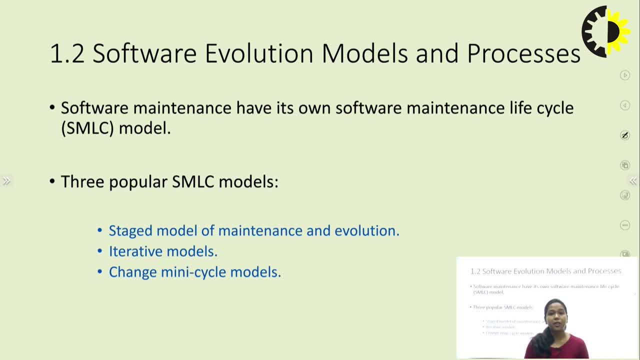 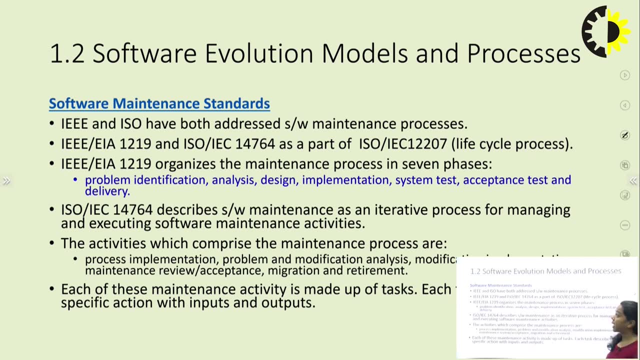 last one is the change mini cycle model. so these are the three different models will going to be used for the software maintenance life cycle software maintenance standard, that is, ieee and the iso have both address the software maintenance process. the ieee, eia 12, 19, the iso as a part of the iso iec 12. 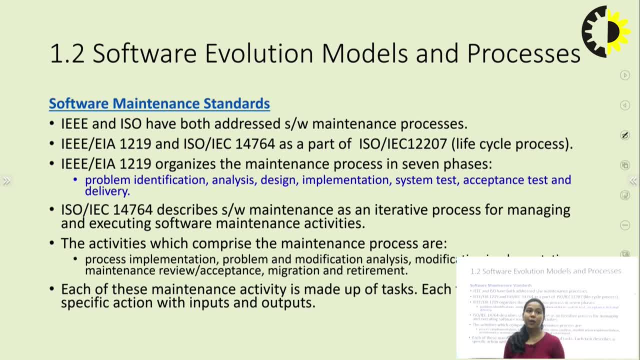 207. these are the recycle process to be performed. so the ieeeia organize the maintenance process in the seven different phases. what are those? the problem identification analysis, designing, maintenance system testing, acceptance testing and the delivery. so iso describe the software maintenance as the iterative process for managing and executing the software maintenance activity. 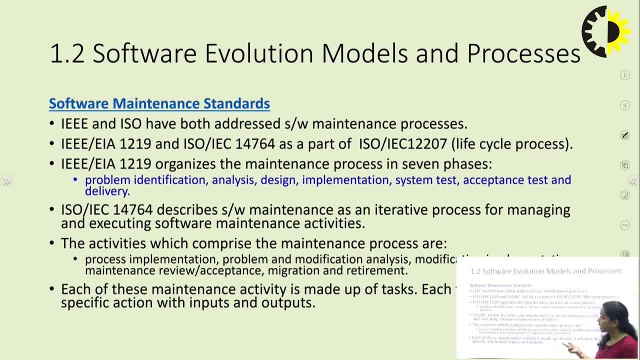 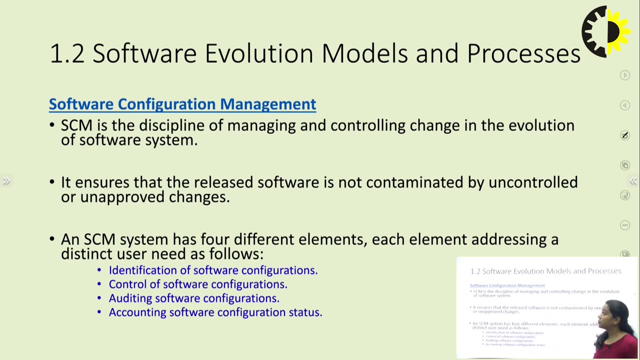 so the activity which comprises the maintenance process are the process implementation, problem modification, analysis, modification of in implementation, maintenance of the review and the retirement. so each of these activity are come under the task of the maintenance. now the next is a software configuration management. as we know, the configuration is a discipline of 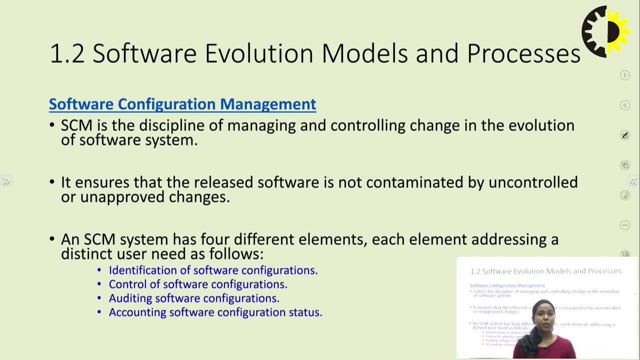 managing and controlling the changes of the evolution of the software system. it ensured that the release of the software is not continuous or by uncontrolled or unapproved changes. So the software configuration management system has a four different elements: Identify the software configuration, control the configuration, audit the software configuration and finally, 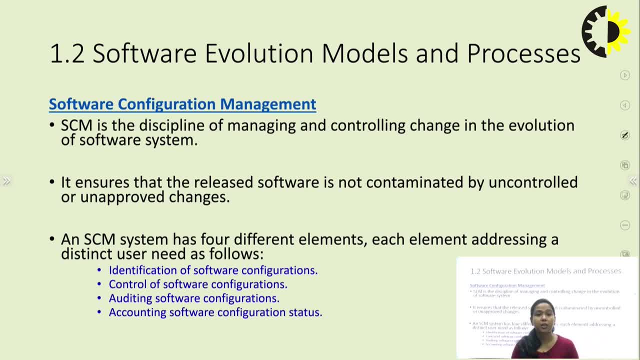 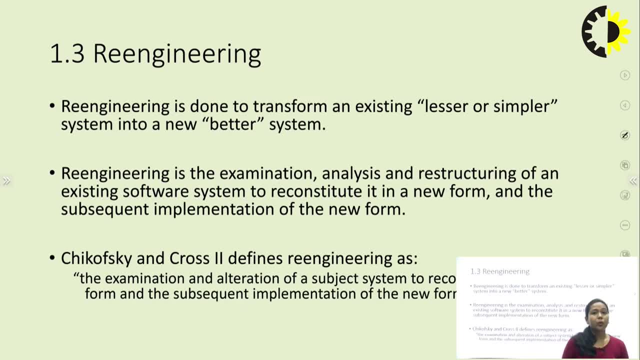 accounting them? the software configuration: What are the different changes to be accumulated in a software as per the evolution? come Now, the next topic we will going to cover, that is the re-engineering. What re-engineering is? Till date, we discussing about the software engineering, but still now we 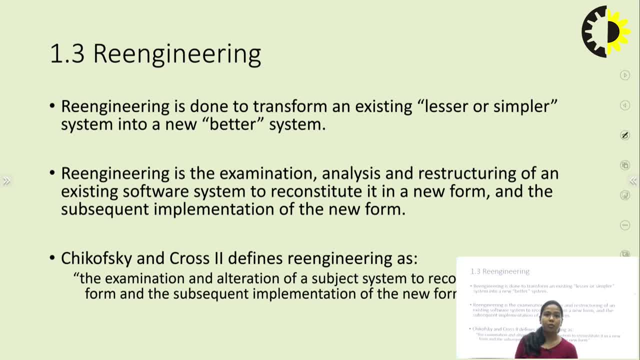 are not at the phase. what re-engineering? the reverse of the complete software engineering, is known as the re-engineering. How it will going to be better as compared to the software engineering. What are the requirement? Why the terminology: come in a market to get advantage of this. So the re-engineering. 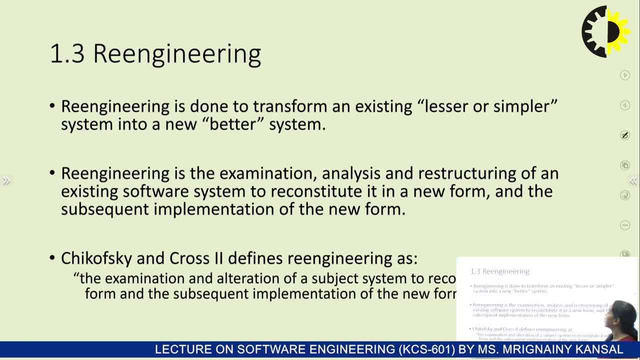 is done to transform an existing, lesser or simpler system into a new, better system, It will reach to the better system. So re-engineering is the examination, analysis and re-constructing of an existing software system to reconstitute in a new form and subsequent implementation of the 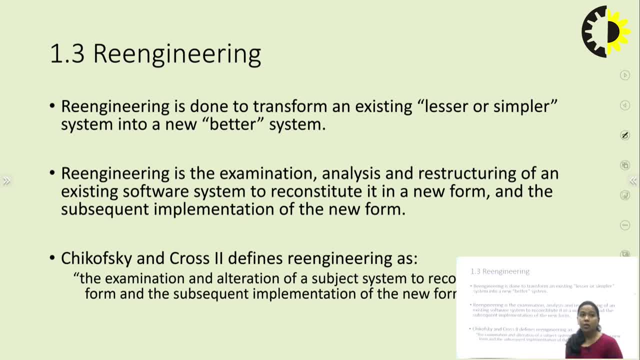 new, different form that is known as the re-engineering. So the Ceskiosii X2 define the re-engineering as the examination and the alteration of the subject system to reconstitute in a new form and subsequent implementation of the new form that is known. 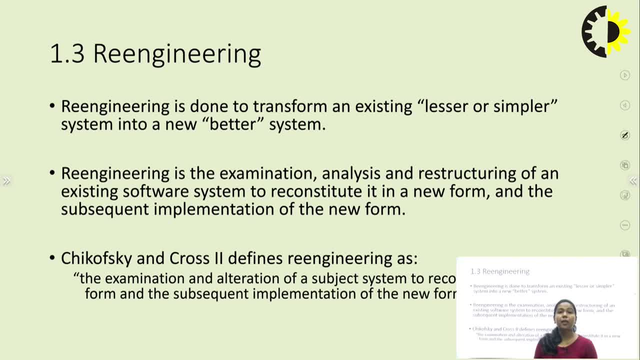 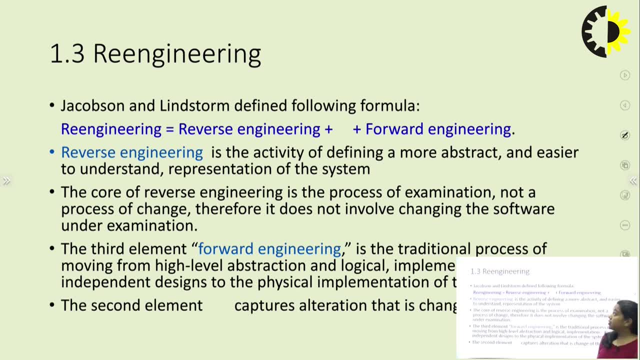 as the definition given by the Chesky and Cross to that what the reengineering is. So Jacobson and the Lindstrom define the formula of the reengineering. that means the reverse engineering plus the forward engineering will make a reengineering. What the reverse engineering is is the activity of defining more abstract and easier to understand. 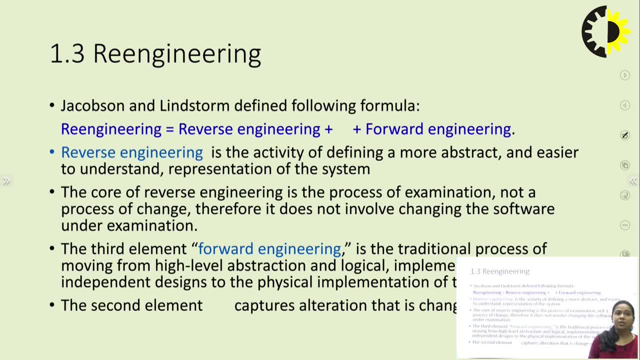 representation of the system. The core of the reverse engineering is the process of examination, not a process of change. Therefore, it does not involve the changes of the software under the examination. So the third element, that is, the forward engineering, what is that? it is a traditional. 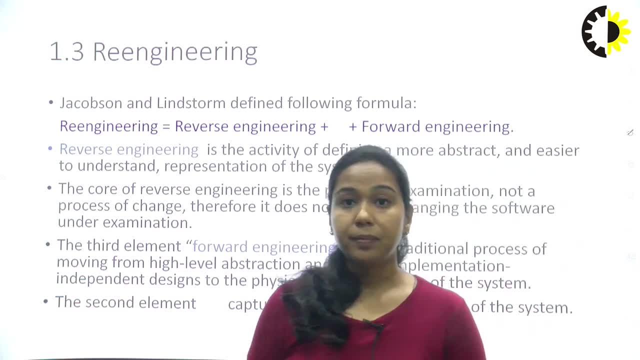 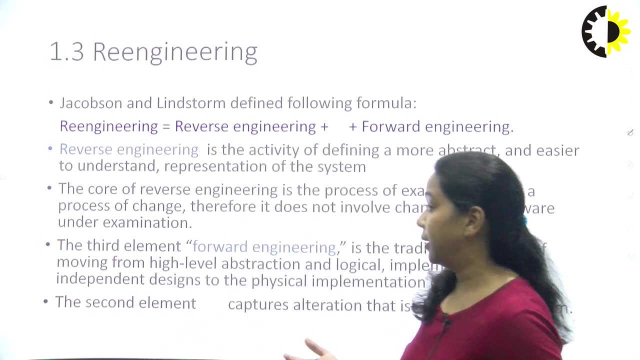 process of moving to the higher level abstraction. That means the traditional way, the way of we are performing The software engineering with the help of the SDLC cycle. So that will be given by this designer, or the physical implementation of the complete system. 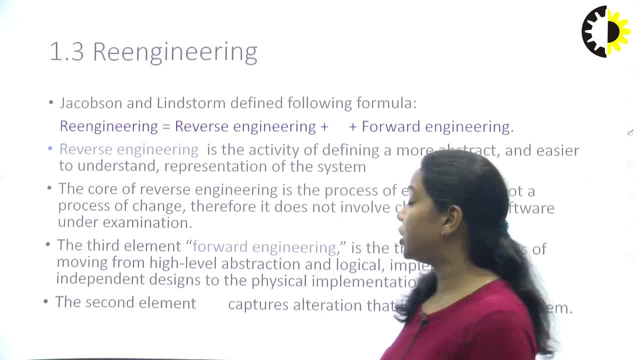 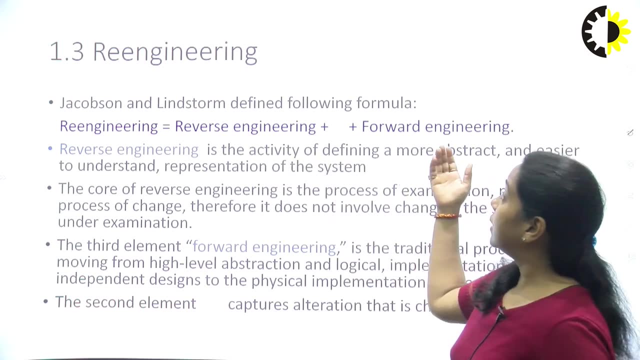 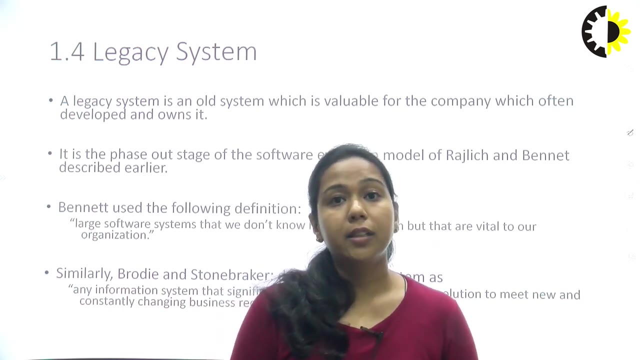 So the second element, character, the alteration of the changes of the system, and this is within the complete definition of the reengineering. that means the reverse engineering and the forward engineering. Now the legacy system, what the legacy system defined. while we are discussing about the 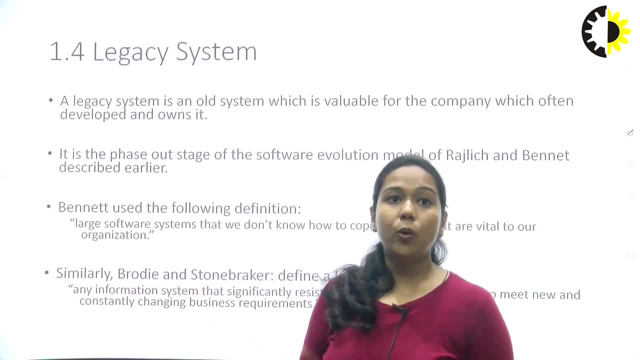 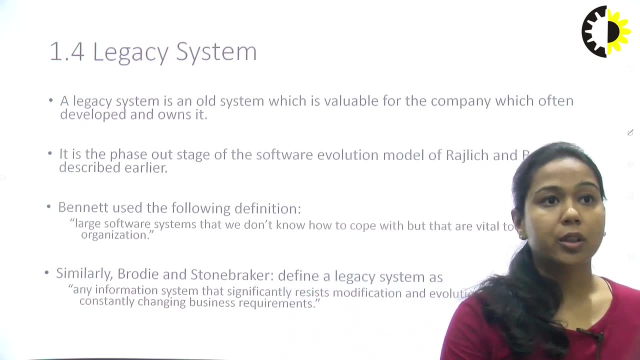 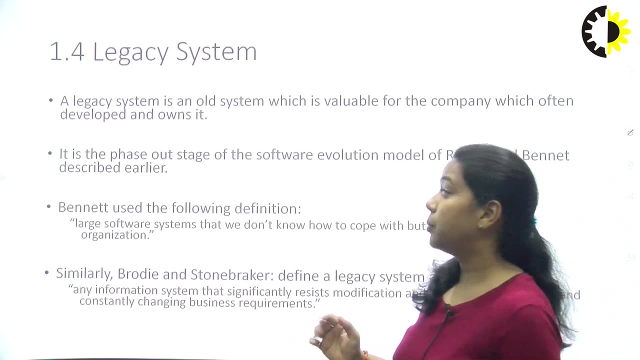 maintenance or the reengineering. So the legacy system. The legacy system is a old system which is valuable for the company, with often the developer and owns it. It is a phase out stage of the software evolution model of the Richlet and the Bennett described. 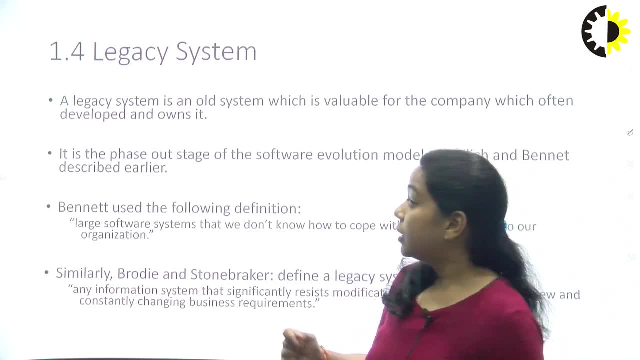 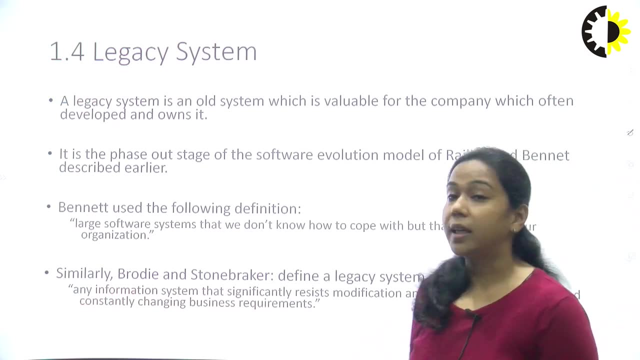 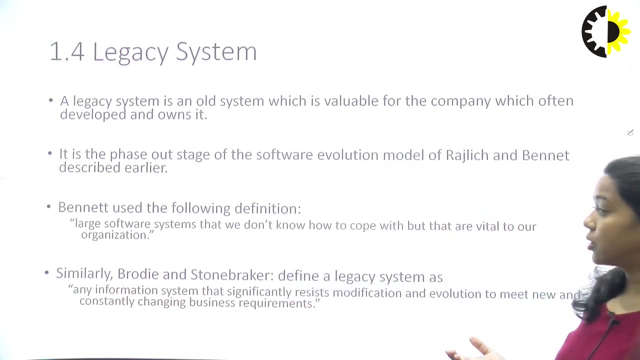 earlier The Bennett used the following definition: that large software system that we do not know how to cope with, but they that are vital of our organization. that is known as the legacy system. That is, the default system of our company. Similarly, the Brock tree and the stone baker define a legacy system as any information. 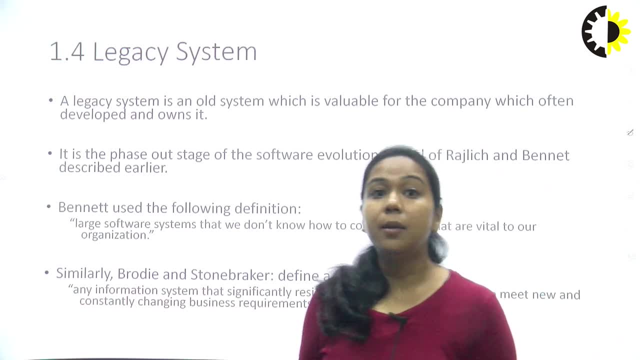 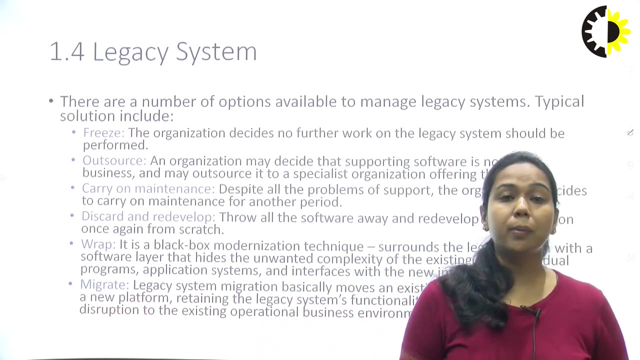 system that is significantly resist the modification of the evolution to meet the new, consistently changed business requirement. that is known as the definition given by the legacy system. There are number of options available to maintain or to manage the legacy system, typically solution given by these. What are those? 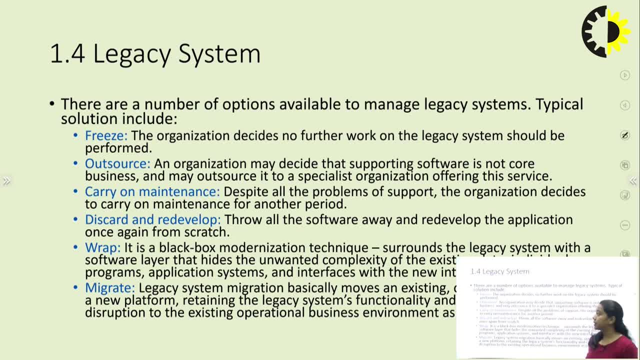 First is the freeze, outsource, carry on maintenance, discard and redevelop, wrap and they migrate. So these are some of the options available for to manage the legacy system, the old system of our company, and to manage them and to maintain them over future. 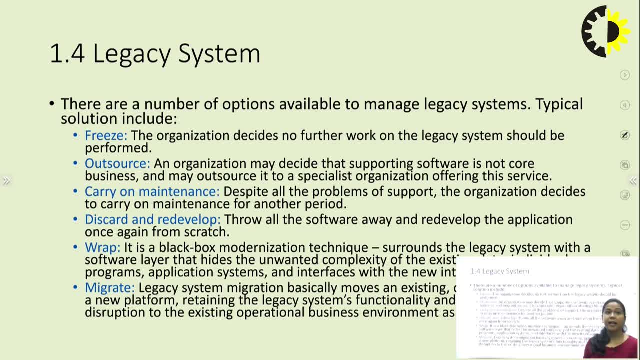 So freeze The organization. decide no further work on the legacy system should be performed. outsource: An organization may decide that supporting software is not the core business and not or may outsource, So outsource it to the specialist organization offering this service, despite of all the problems. 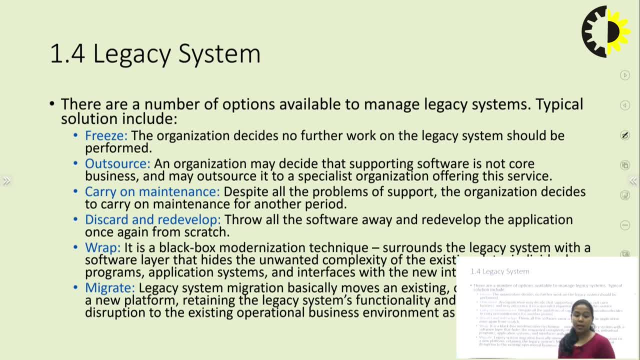 and support that the decision to carry the maintenance for an another period, Discard and redevelop, throw all the software away and redevelop the application once again, for from the scratch The wrap. it is the outbox. Outbox of modernization techniques, surrounded the legacy system with the software layout. 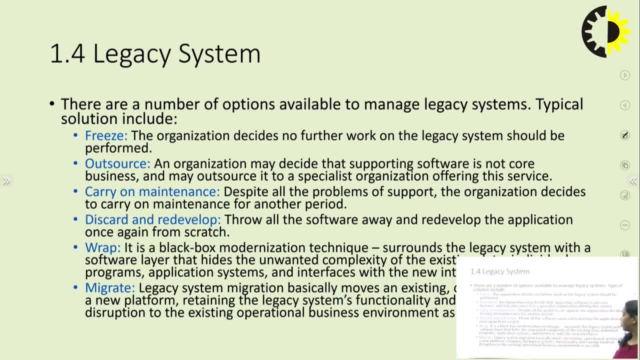 layers and applications Layers and hidden the unwanted complexity of existing data. Individually. the program will come into the maintenance phase and interact with the new requirement. Migrate that the legacy system migration basically move an existing operational system to a new platform to make it in a new way to manage them and to run them by the user. 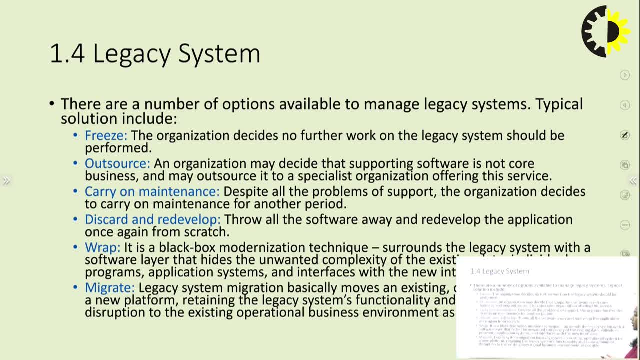 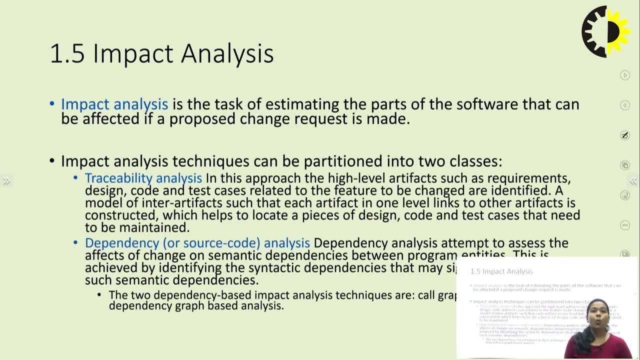 So retaining the legacy system functionality and causing the minimal disruption to the existing operational businesses, An activity using the data to make it more efficient and the environment as much as possible. What are the different impact analysis over the doing the maintenance of a software? 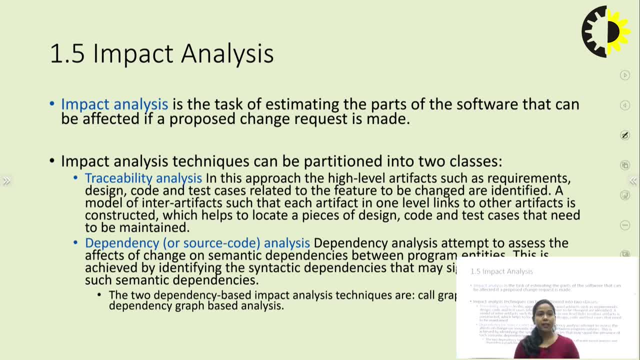 So impact analysis is a task of eliminating the part of the software that is affected by the proposed size change requesting is made. So impact analysis technique can be partitioning into two different classes: First of all, the traceability analysis and second is the dependency- how they are actually. 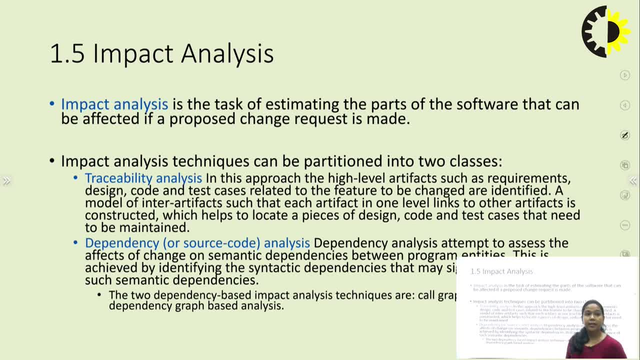 depending on two different classes How this works. you can also do the same with the other claims. Let us now move towards the application. So traceability. In this approach, the high-level artifacts, such as requirement, design code and test cases related to the feature to be changed and identify the model on the inter-artifacts, such as each artifact is one level link to other artifact and it constructed with the help of the locator of the piece of design of code. test and maintain them. 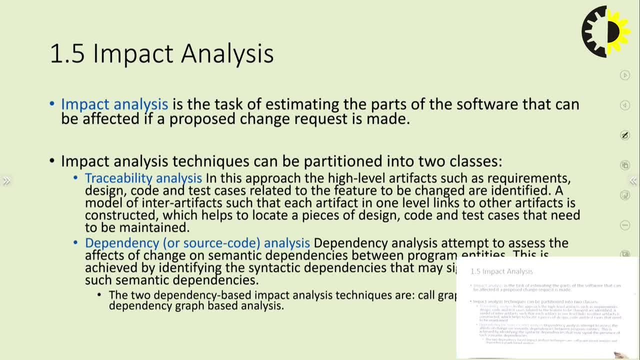 Dependency. Dependency analysis attempt to access the effect of change on the semantic dependencies between program entities. This is achieved by identifying the semantic dependency that may signal the presence of such semantic dependency. So there are two different dependency-based impact analysis techniques: Call graph-based analysis and the dependency graph-based analysis. These are the two different dependencies to be there. 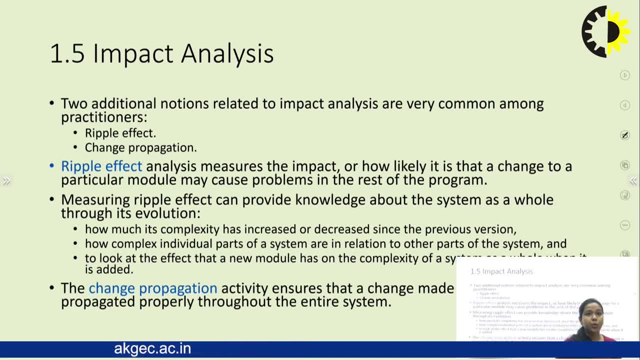 All the traditional notation related to the impact analysis are very common among the practitioner. What is the effect? are those ripple effect and the change propagation? What is the ripple effect? It analyzes the misa of that. how likely to be change a particular. 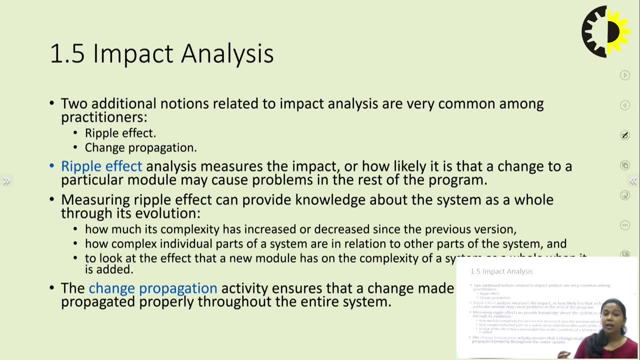 module and may cause the problem in the rest of the program. How, if I am changing one module, then how it will going to be change or effect the complete system or complete program. So measuring of this ripple effect can provide a knowledge about the system as 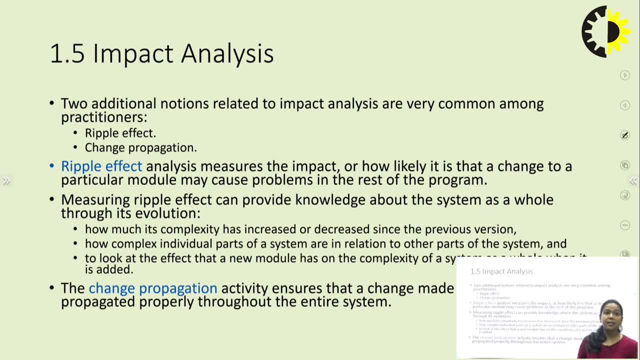 a whole help of the evolution, How much it complexity has increased and decreases on the basis of the previous version, How the complex individual part of a system are in the relation to the other part of the system and it also take took effect. 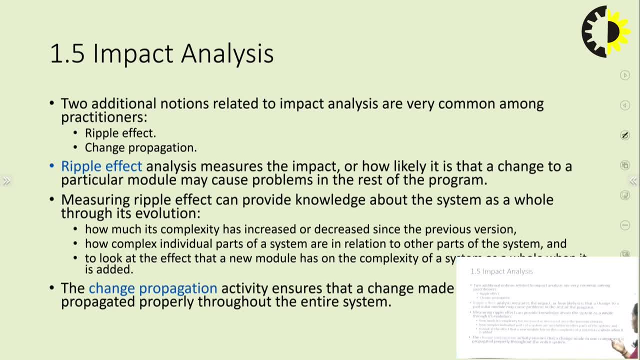 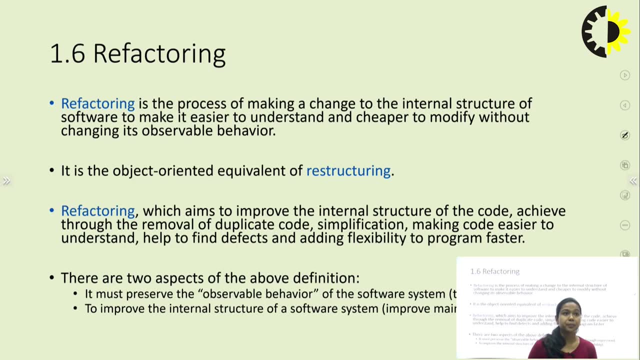 of the new modules based on the complexity system as a whole, when it is going to be added The change propagation activity, ensuring that the change made in one component propagate properly throughout the entire system. that is known as the change propagation effect. Now the next terminology that is known. 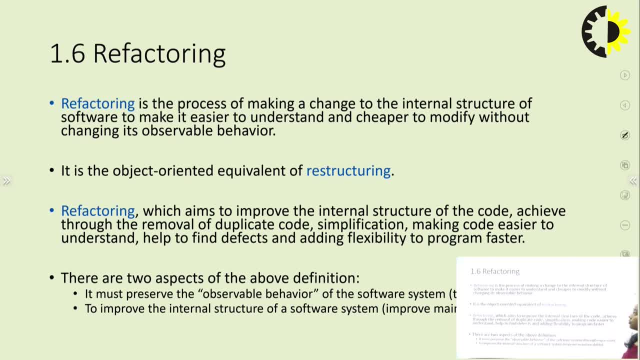 as the refactoring. Refactoring is the process of making a change to the internal structure of the software to make it easier to understandable, to cheaper for the whole change to be, without changing any behavior or the operation or observable behavior of the system. Then we perform the changes. 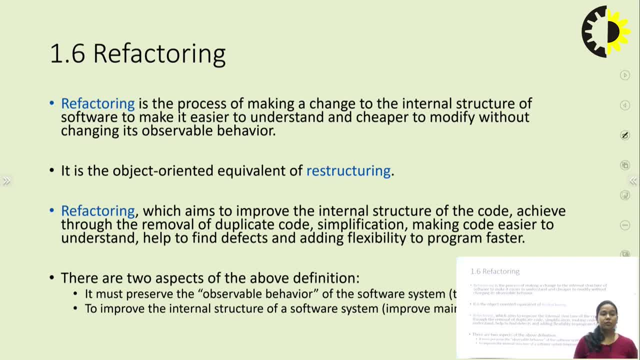 internally, It is the object-oriented evaluant and the re-property Structuring Refactoring, which aim to improve the internal structure of a code through the help of the removal of duplicate code, Simplification, making code easier to understand, help to find the defect and adding it to the 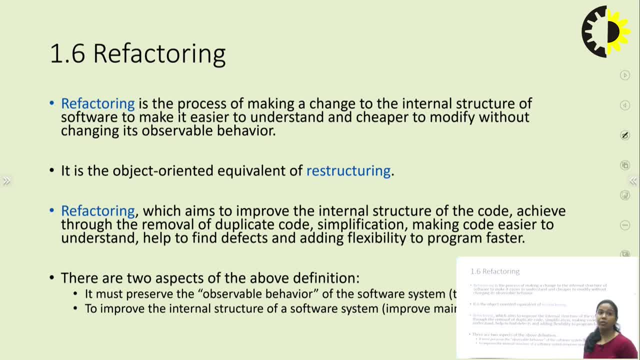 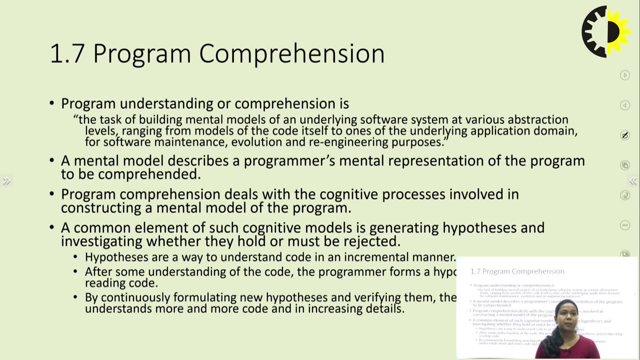 flexibility. There are two different aspects of the above definition: that it must preserve the observable behavior of the software system and it also improve the internal structure of the system software. So these are the two different aspects to be recognized by the software. Next is the program comprehension, Program understanding and the 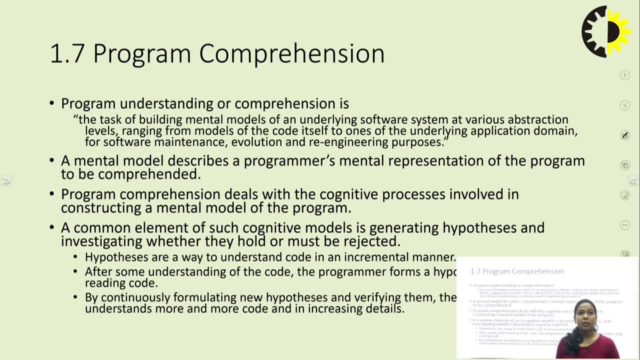 comprehension is a task of building the mental, mental model and underlying the software system for the various abstract level, ranging them for the model of a code, itself one of the underlying application domain for the software maintenance evolution and the re-engineering to be performed. So a 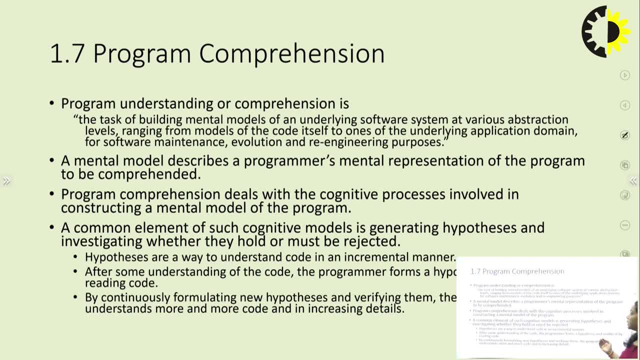 mental model describe a programmer mental representation of a program. to be comprehensive, The mental state at which state will going to be programmer will code the complete program. So the program comprehension deal with the consecutive process involved in constructing a mental model of the program. A common element of such consecutive model is: 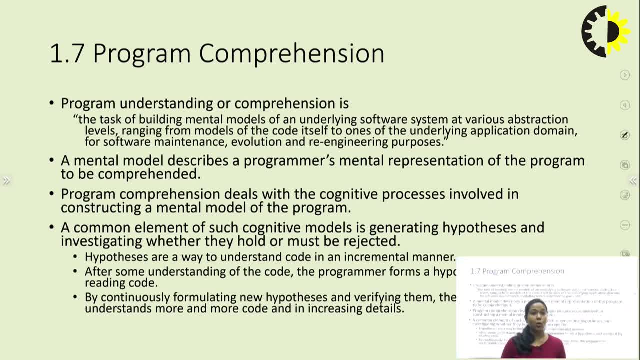 generative hypothesis and investigate that, whether they are holding this or rejecting this Hypothesis, are the way to understand the code in the incremental way. After some understanding of the code, the programmer form a hypothesis and verifying it to reading code By continuing the formulated of new hypothesis and 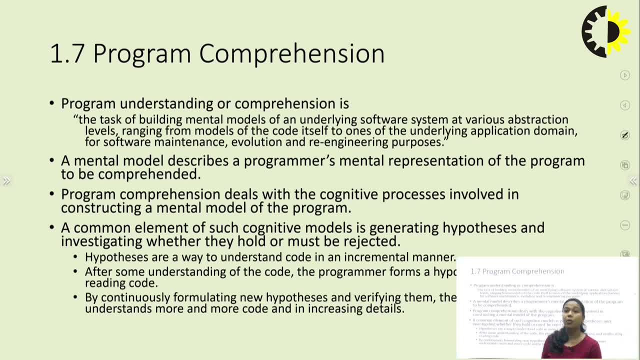 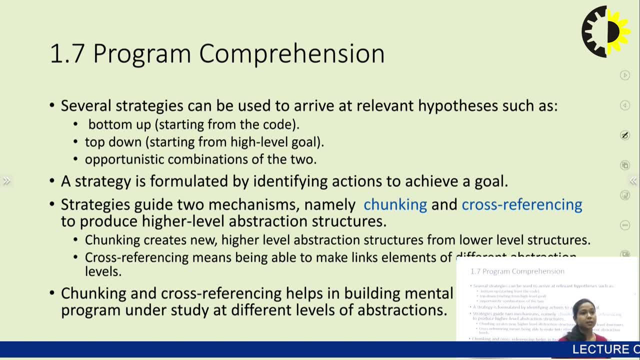 verifying them. the programmer understand more and more code in the form of increasing way, Several different strategies to be perform while doing the hypothesis, that is, with the help of bottom up, starting from the code, top down, starting from the high level goal and the opportunistic combination of the two. 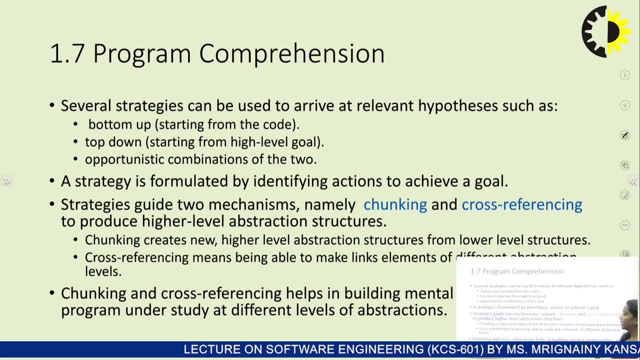 different approaches. So the strategies formulated by identifying the action of achieving a goal These strategies guide into, namely as to that is the chunking and the cross referring to produce the high level abstraction structuring. So the chunking create the new high level abstract and the cross referring means able to make 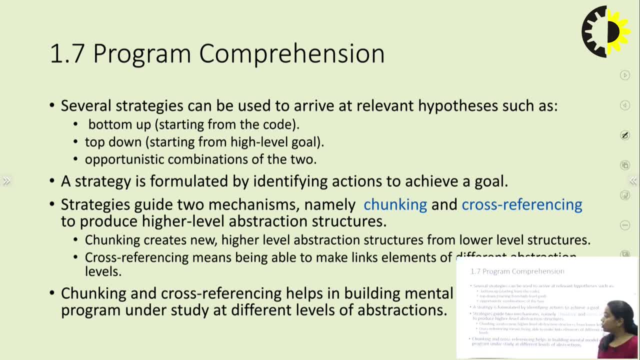 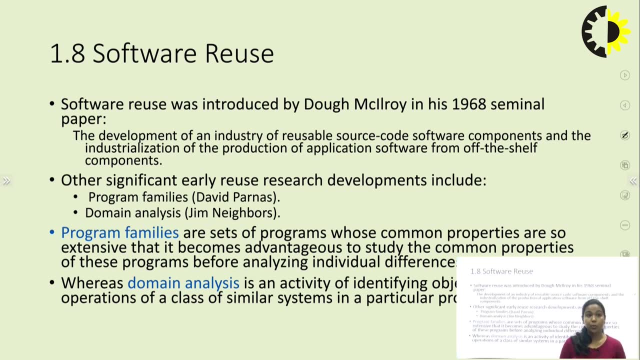 the link element of the different abstraction level. So chunking and cross referring help in building a mental model of program under ال application software from the off of the shelf component. So other significantly using the off-of-the-shelf application software is called creative processing, Cuz area left and individual. 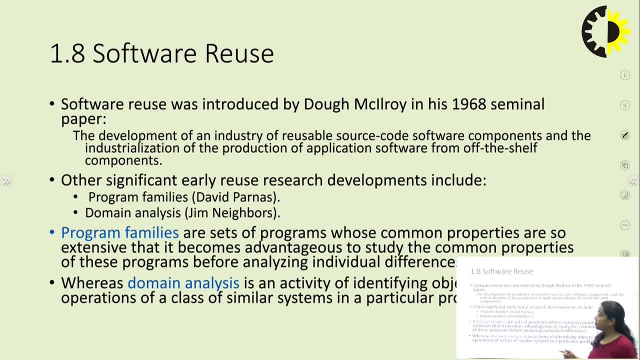 and from the expression of our purpose, as before, Software task performance and MortalымиWhen we designed, we have certain components, like kind ofonents flow adventurers, reusable by the help of the program families and the domain analysis Program families, that is, a set of program, that whose common properties are so 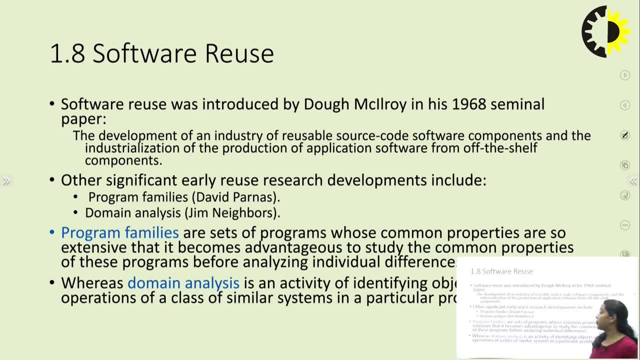 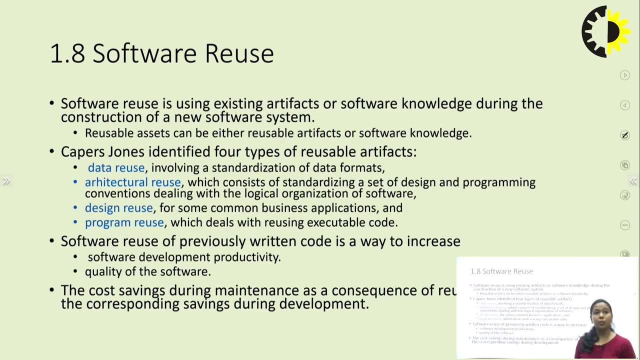 extensive that it become advantages for the study of the common properties, as these program before the analyzing an individual difference. Whereas the domain analysis is an activity of identifying the object and operations of a class of similar system in a particular problem and the domain This reuse is using to 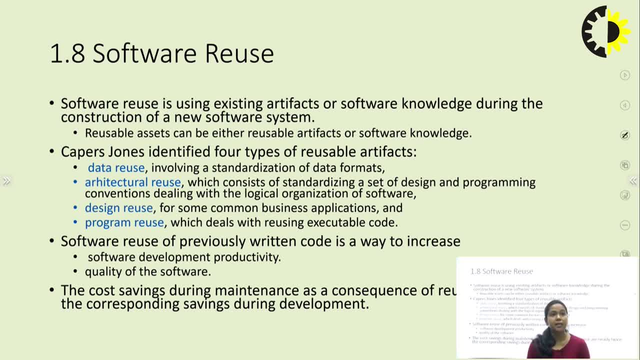 existing, the artifact of the software knowledge. during the reconstruction of the new, different software, This reusability- that means a common code, source code- can be easily used for the another program to be developed, which will reduce the time of developers, reduce the cost and easy deliver to the.